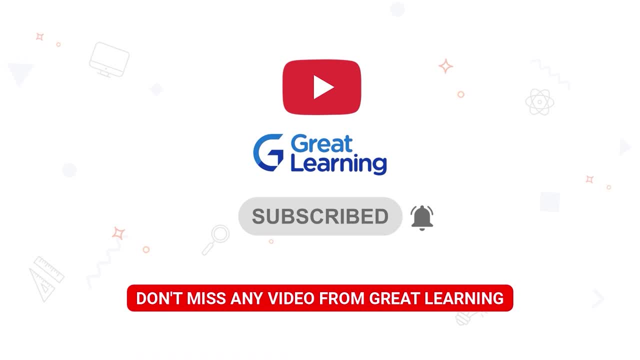 and turn on the notification bell so that you receive as soon as we post a new video. Thank you so much for watching this video. you don't miss out on any new update or video releases from great learning. if you enjoy this video, show us some love and like this video. knowledge increases by sharing, so make sure. 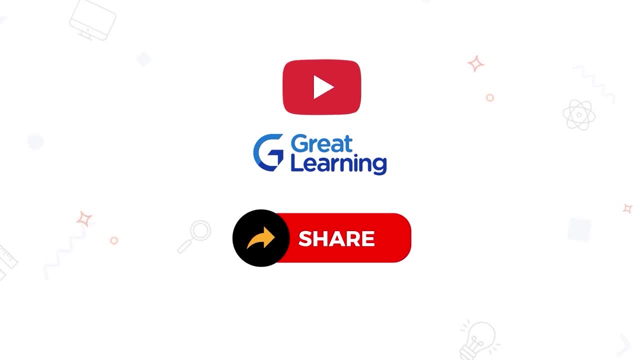 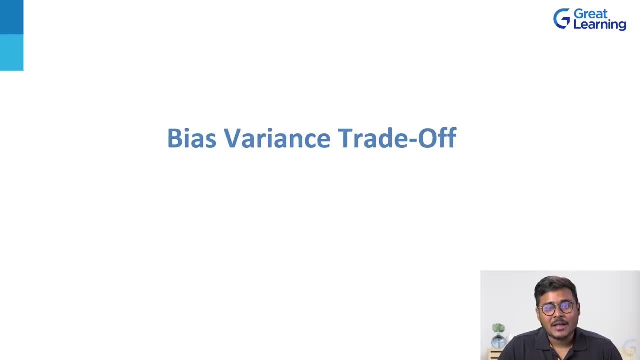 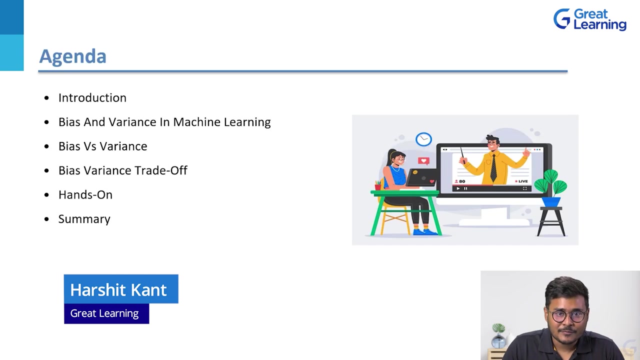 you share this video with your friends and colleagues. make sure to comment on the video for any query or suggestions and i will respond to your comments. hello everyone. today i'll be talking about the topic bias- variance trade-off in machine learning. so let's just look at the agenda for. 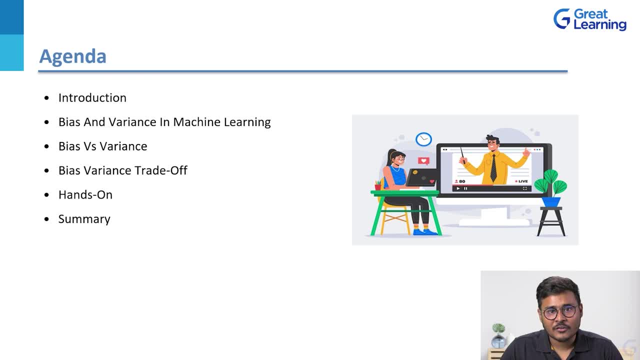 today. i'll be starting off by giving you a general introduction through a small example. then i'll move on and talk about bias and variance in machine learning further, which i'll be talking about bias versus variance like. what are the distinctive differences between these two whenever we talk? 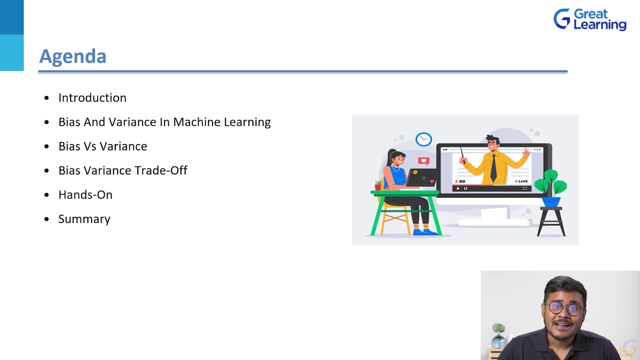 about bias and variance in a machine learning model, then i'll be showing you a hands-on using a data set on google colab, and then i'll be ending this presentation by summarizing all the points. so let's move on and dive right into the first part, which is the introduction. 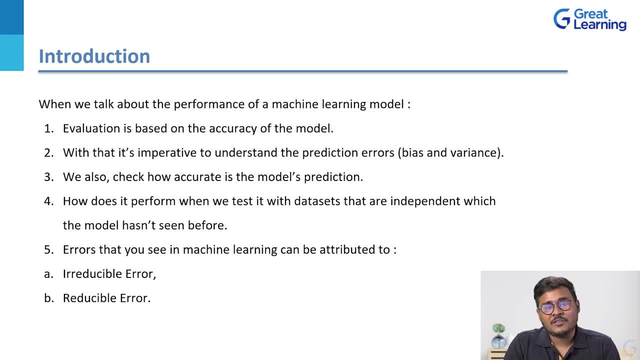 now, whenever we talk about the performance of our machine learning model, we generally divide it into these pointers. evaluation is always based on the accuracy of the model. with that it also becomes imperative or important to understand the prediction errors right. so whenever we are doing evaluation based on the accuracy of how your machine learning model is going to perform, 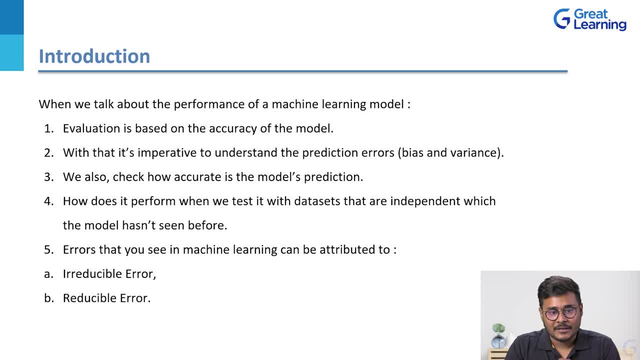 we also check: how accurate is your model's prediction right like, for example, how does it perform when we test it with data sets that are independent, you know, data sets that your model has never been seen before, or data set which are which your model has never been tested on before. 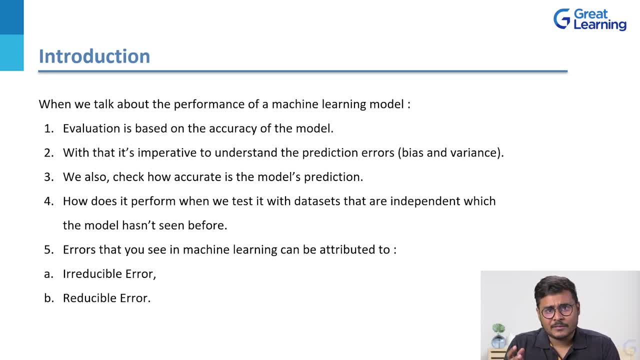 right, and then we also talk about errors. so, basically, whenever we talk about errors in machine learning, there are two kinds of them. one is the irreducible error and the second one is the irreducible error. so let's move ahead and understand what is irreducible error. 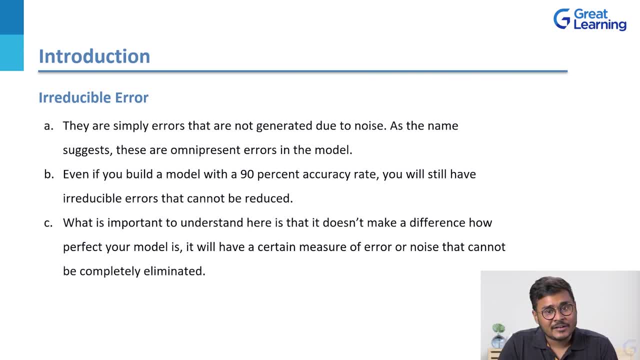 now. irreducible errors are simply errors that are not generated due to noise, as the name suggests. these are errors which are omnipresent throughout your model. now, let's say, even if you are a machine learning engineer or a data scientist who's working in a company, you developed a machine. 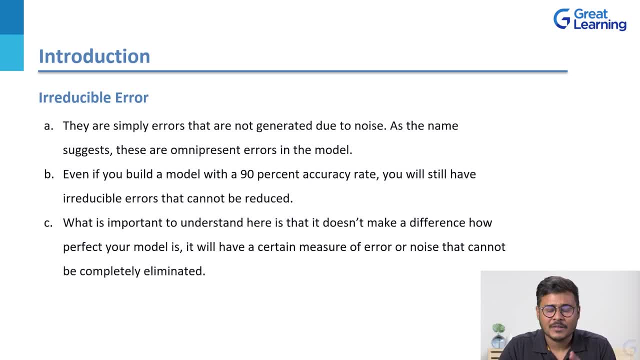 learning model and the accuracy rate of your model is around 90 percent, you will still have irreducible errors throughout your model. what is very important here to understand is that it doesn't make a difference how perfect your model is, even if your model is extremely perfect and it performs. 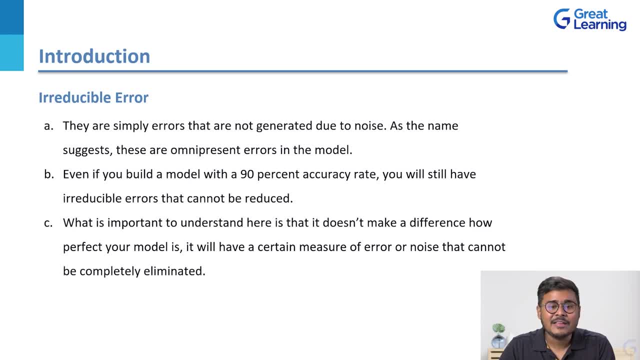 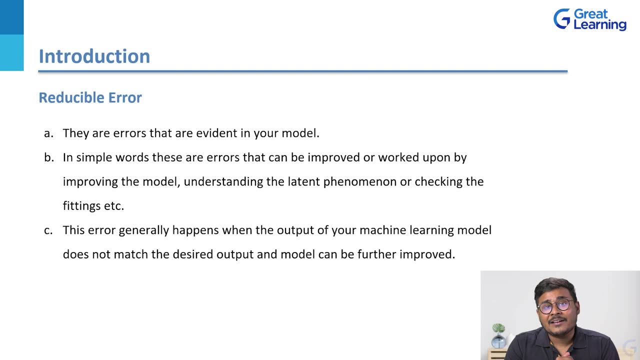 really well on all the parameters, it will still have a certain degree or a measure of error or or noise that cannot be eradicated or removed. so this was about irreducible error. people. let's move on and i'll be explaining you about the reducible errors now. reducible errors are errors which are: 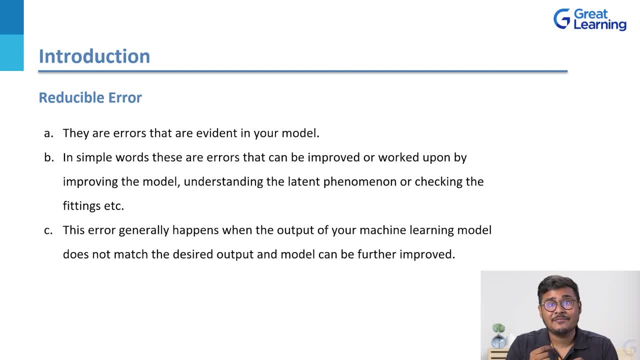 present in your model. when we spoke about irreducible errors, these are basically very small errors which you don't actively see in your model, but they are present. reducible errors are errors which you actively see in your model. right in simple words, these errors can be improved or worked upon. 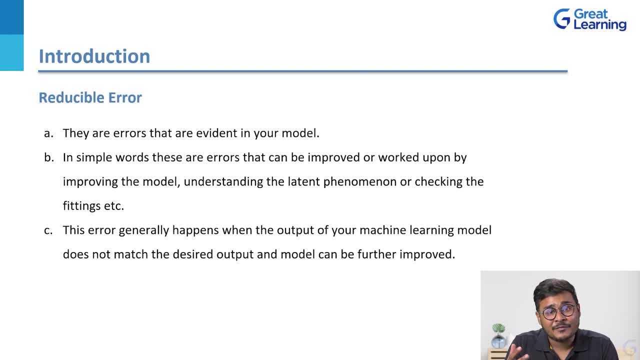 by improving the model, for example, understanding the latin phenomenon, how your model is performing, or checking the fitting: does your model have any sort of overfitting or underfitting, etc. this error generally takes place or happens when the output of your machine learning model does not match the desired output and model can. 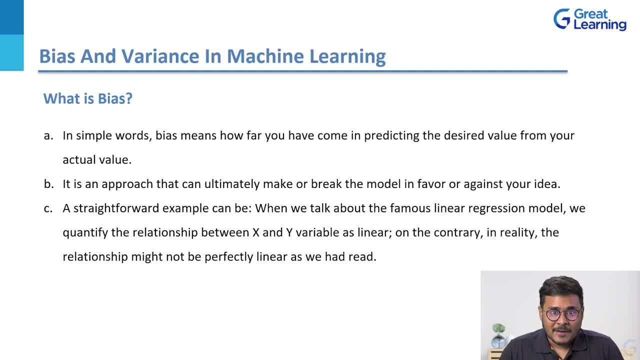 be further improved. so now let me start off by explaining you what is bias under the topic bias and variance in machine learning. in simple words, bias means how far you have come in predicting the desired value from your actual value. well, it can also be thought of as the ultimate approach which can break the model in favor or against your idea. 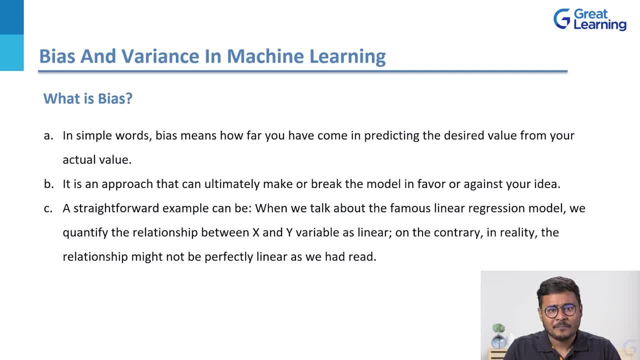 now, what do i mean by this entire statement? how far you have come in predicting the desired value from your actual value? well, it generally happens as that, in your entire journey of your machine learning engineer or a data scientist, you would be building machine learning models. right now, here, the decisive factor would be: how will you be able to measure the desired value? 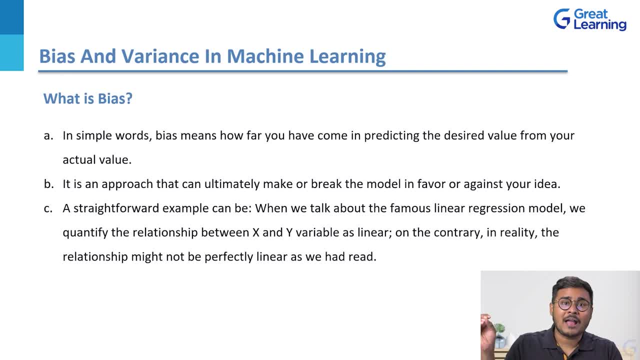 that is the desired machine learning model that you wanted from your actual value, that is, the data trained it on, or the problem statement, which is it which it is based upon. now moving forward, one of the straightforward example of this can be your linear regression algorithm. now we 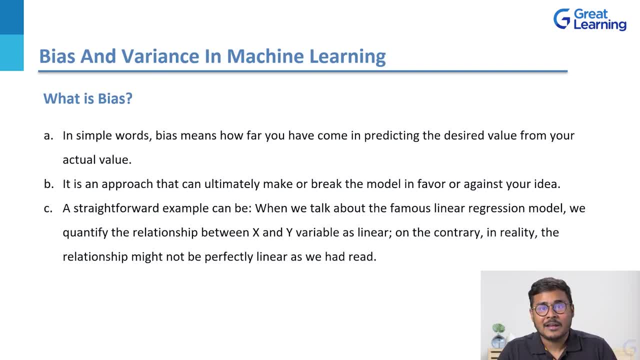 all learn about linear regression algorithm when we start our journey in machine learning, right? so we basically try to quantify the relationship between two variables, x and y, as linear. on the contrary, in real life, it just so happens that the relationship between these two variables are not party linear and relative to linear lord, they shouldn't be around linear, linear. 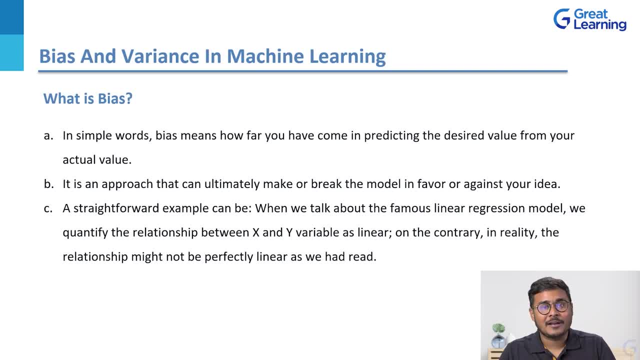 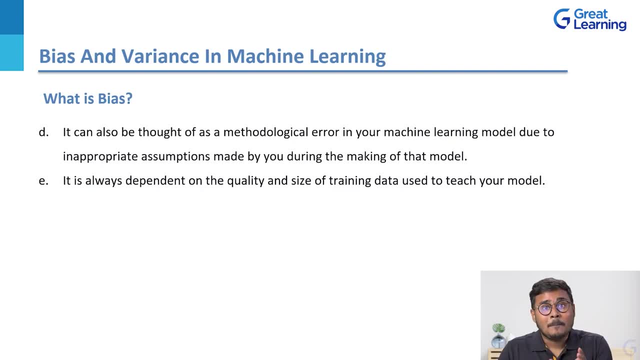 perfectly linear, So what we had read in textbook or wherever we had read the source from it cannot be entirely correct. So what is this particular term bias? It can be thought of as a methodological error in your machine learning model due to inappropriate assumptions made by you during. 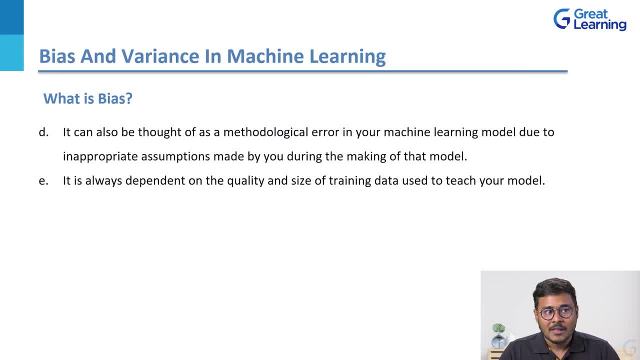 the making of that model. Now, what do I mean by this entire statement? Well, it is some sort of an error right Now when I say these two words inappropriate assumption. what I basically mean is: these assumptions can stem from various reasons. It can be a human, cognitive assumption, or it can 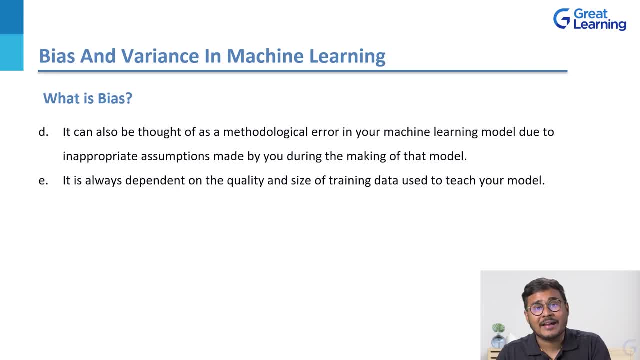 be an error in taking some sort of a survey or while you are collecting data. It is always dependent on two parameters, one being the quality and other being the size of your training data set that you are using to teach your machine learning model. Now let's move ahead and 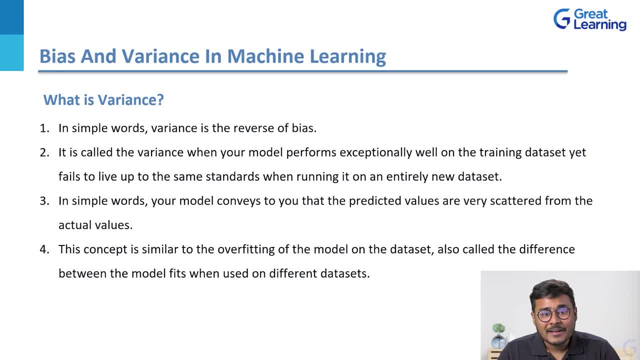 understand the difference between a machine learning model and a machine learning model In very simple words: variance is the reverse of bias. It is called variance because here your model performs exceptionally well on the training data set right, Yet it fails to perform on the 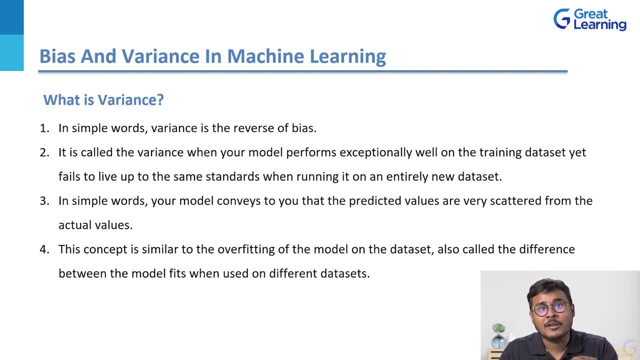 same level when you train it or when you introduce a new data set right? So, in simple words, your model is trying to convey you that your predicted values are very far away or scattered from your actual values. This concept is also similar to a concept called overfitting of model on the data set, which is 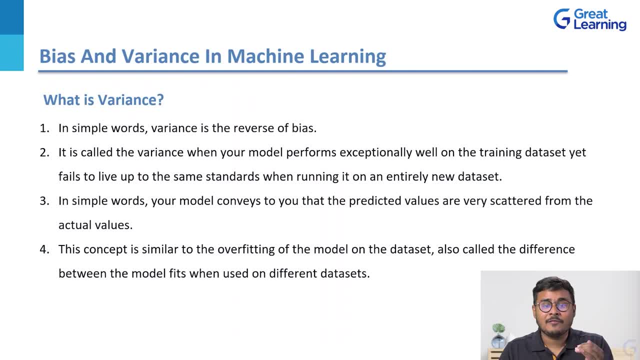 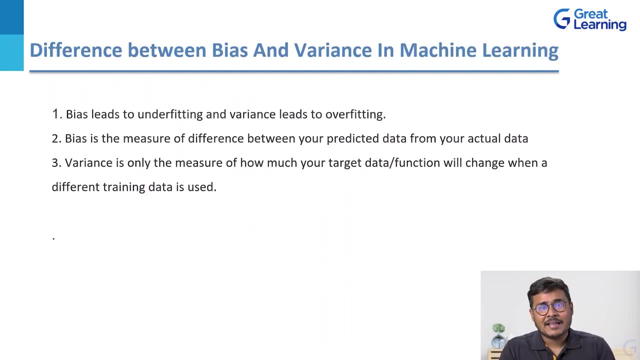 also called as the difference between the model fits when we are using it on different data sets By different data sets. what I mean here is your usual training data set and an entirely new training data set. Now let's move ahead and understand few differences between bias and 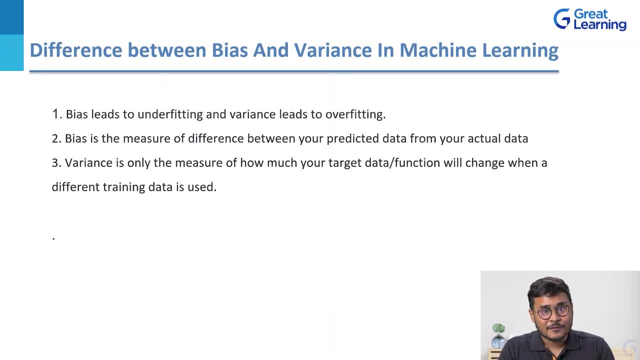 variance in machine learning. Well, bias leads to underfitting and variance leads to underfitting. This leads to overfitting of the data. We'll be learning about these two particular terms further ahead in the presentation. Bias is also the measure of difference between your predicted data from 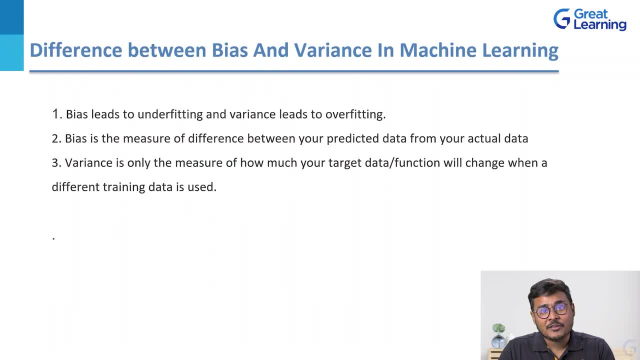 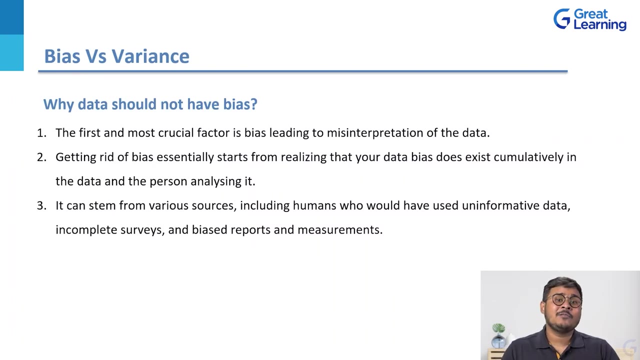 your actual data. However, variance is only the measure of how much your target data or your target function will change when you run it on an entirely new training data set. Now let's move ahead, where I'll be talking about bias versus variance. So here I'll be discussing one of the 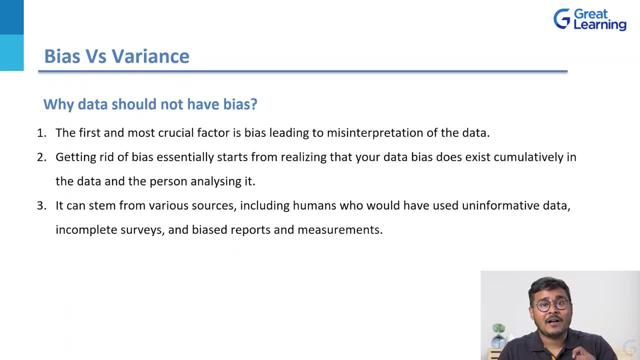 important parts: why your data should not have biases, or why your data should not have bias. What is the reason of having it? The first and the most crucial factor to understand here is that bias leads to misinterpretation of your data. Getting rid of bias essentially starts from you. 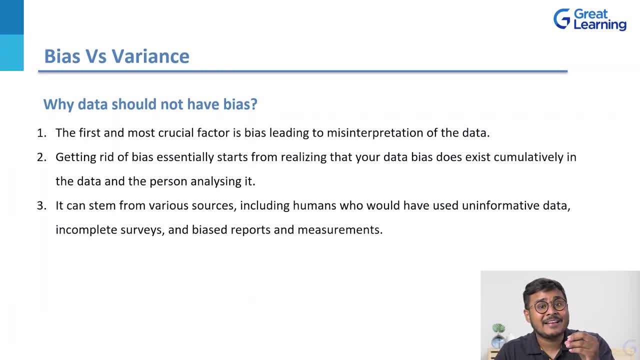 that is a stage where you realize is that you know the bias that exists in your data is not a cumulative factor of the data and the person analyzing it. Now, what do I mean? Now, you can be a person who has done some mistakes or had certain biases. 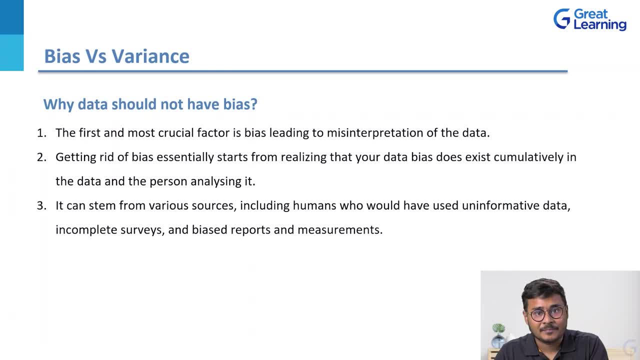 when you were collecting the data or when you were making that data set right, So, and then there could be an inherent bias of the data also, So that you have to realize that you need to separate these two parts apart. The third and the most important point is it can stem from various 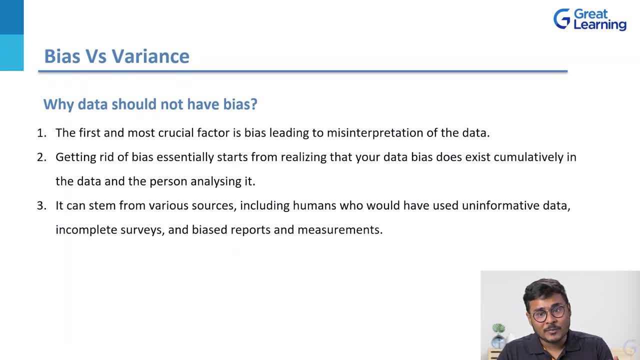 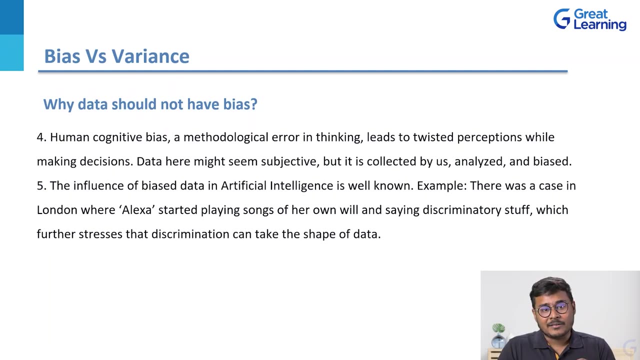 sources, As I had already discussed, the sources include humans who would have used formative data or, you know, incomplete surveys or biased reports and measurements. Other points is human cognitive bias. Human cognitive bias is basically a error. It is some sort of a methodological error or a flaw in your way of thinking or in your way of collecting. 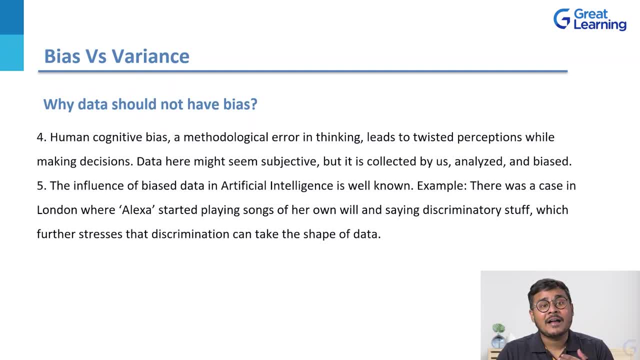 the data right. So basically, it leads to different kinds of perceptions, or I can say twisted perceptions, when you're making decisions, The data here might seem extremely subjective. Now, for example, let me give you a very small example here. You are a data scientist. You are the only data. 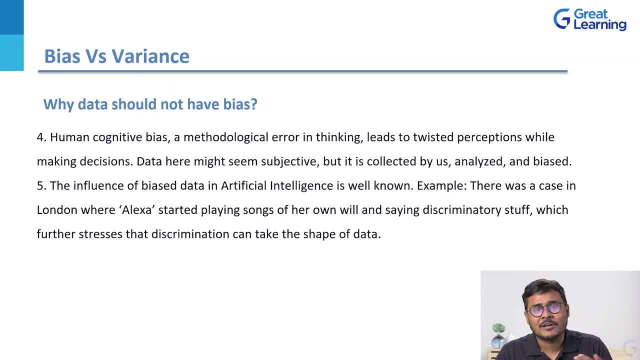 scientist who works in the organization of a certain organization or a company. You have been given a certain task: to make a machine learning model. Now, that model which you're going to make will always have a cognitive bias attached to it, because you will be taking certain 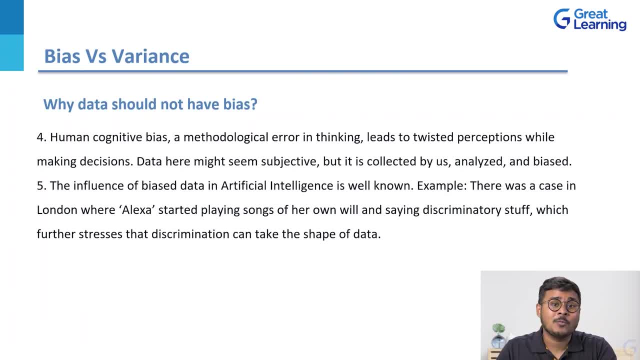 parameters according to what you think is right, But that's not what the organization is looking for when you make your machine learning model. Another point is the influence of this biased data in the world of artificial intelligence is huge. Let me give you an example: how So? there was a case that happened in the year in 2014 in London, where 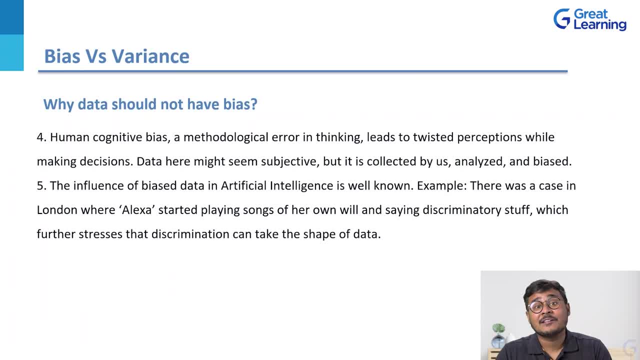 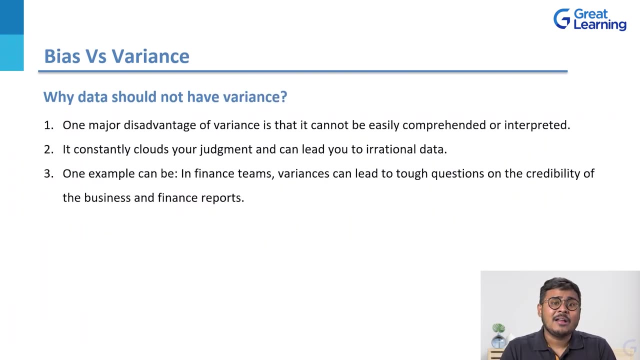 Alexa started playing songs of its own and started saying discriminatory stuff to the person who owned it. Now here, the word discrimination is also some sort of a bias right, Because it takes the shape of the data, and that leads to a lot of flaws. Now let's understand why your data should. 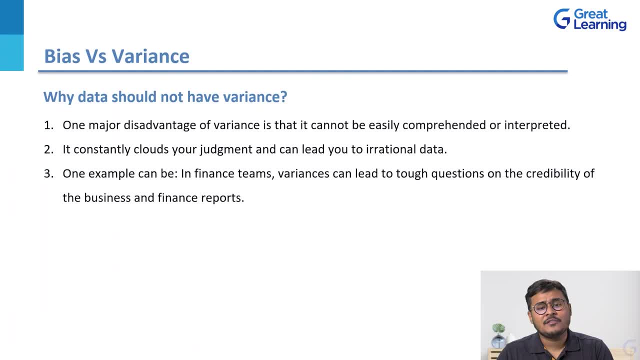 not have variance. One major disadvantage of variance is that you cannot very easily interpret or understand it. It constantly clouds your judgment. What I mean when I say this particular word clouds your judgment is it constantly makes you question your own judgments or your own decisions, which leads to a very messy and irrational data. One example can be in finance. 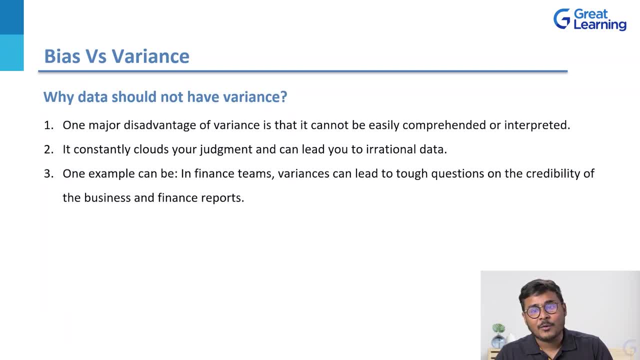 teams. variances sometimes can lead to a lot of flaws, So if you have a very messy data, you cannot very easily interpret it. So let's understand why your data should not have variance. So now let me talk about why your data should not have variance. Now one of the major disadvantage: 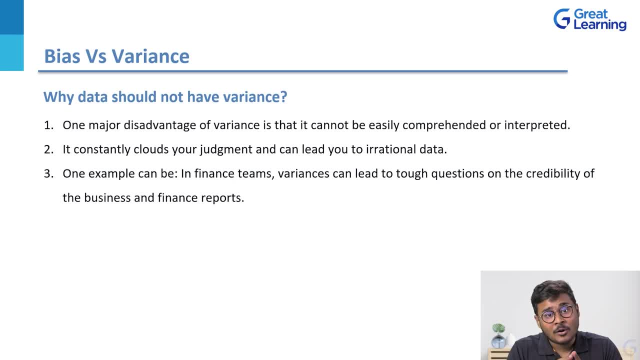 of variance is that it cannot be easily understood or interpreted. It constantly clouds your judgment. Now, what do I mean by this particular term? clouds your judgment? What generally happens is it will force you to question your own decisions, which ultimately leads to messy. 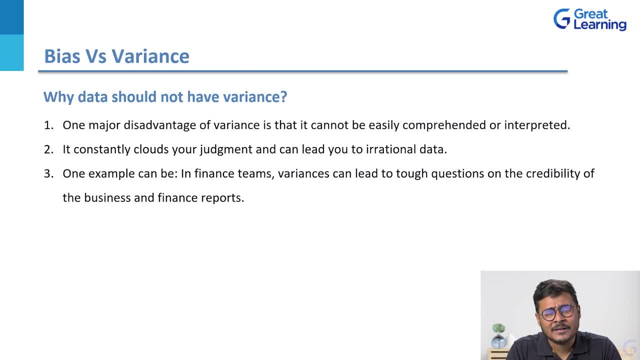 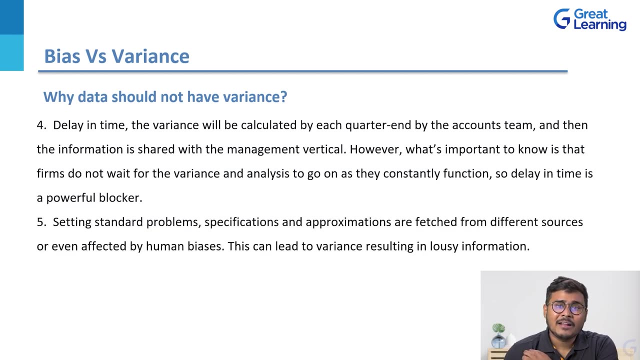 messy and irrational data. One of the most common example can be in finance teams working across different organizations, different companies. variances can lead to tough questions on the credibility of the business and the finance reports. Moving forward, there are 2-3 more steps like this that lead to variance in data. One of them is delaying in time. 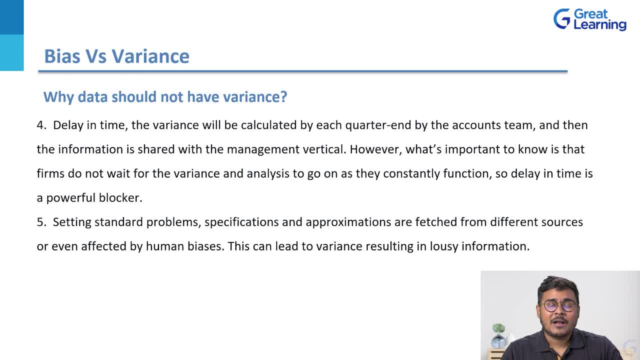 And the example can be again. let's say there is an account team- accounts team- that works in an organization, So the variance is calculated by accounts team each quarter and then the information is shared with the upper management or the other hierarchy. However, what's important? 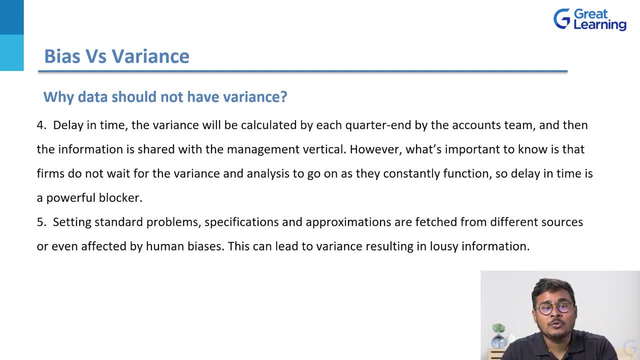 to know here is that firms or organizations do not wait for the variance and analysis to go on, as they constantly function. So delay in time is one of the most powerful blocker which can lead to variances in your data. Again, another point is setting standard. 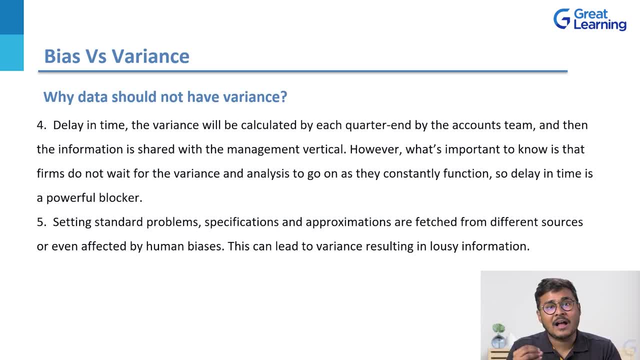 problems. Specifications and approximations are fetched from different sources. So the specifications of the data, or you know, the approximations that people are trying to approximate in the data, they can fetch it from different sources, different areas, and they are also affected by human biases. This can also lead to variance, resulting in lousy or incomplete. 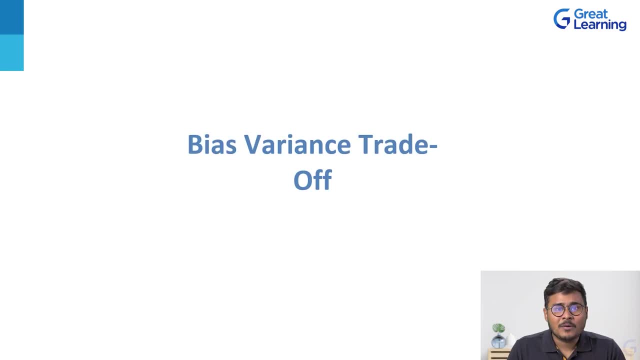 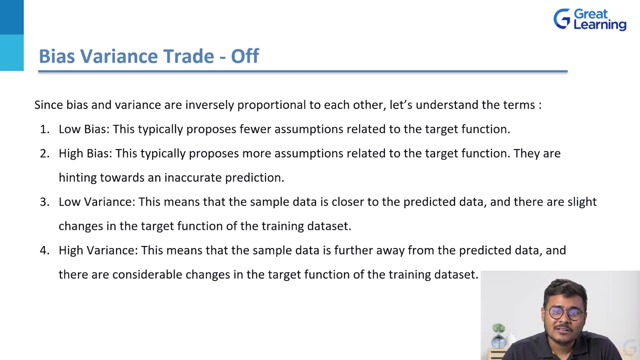 or misinterpreted information. Now let's move forward, where I'll be talking about bias variance trade-off, Since bias and variance are inversely proportional to each other. let's understand the terms low bias, low variance, high bias and high variance perfectly. So what do we mean by? 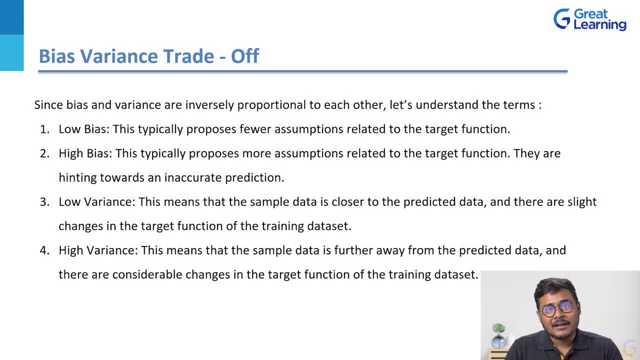 low bias. Well, low bias generally means that it is trying to propose fewer assumptions related to the target function, which is also related to your target data, like the assumptions that you make are very few. High bias means high bias is just the reverse of low bias. 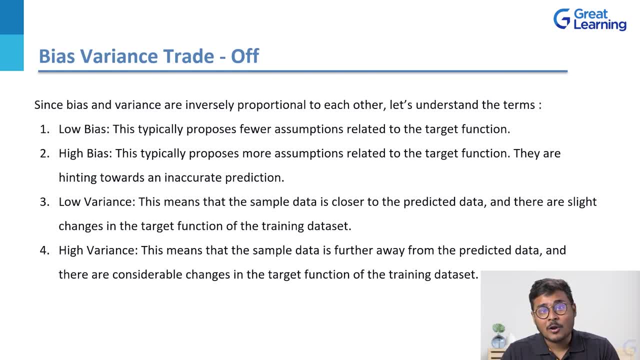 So here it is typically proposing a lot of assumptions to your target function or target data. So, basically, what it is hinting towards is an inaccurate prediction of your data. So what do we mean by low variance? now, Low variance means that your sample data is very close to the predicted. 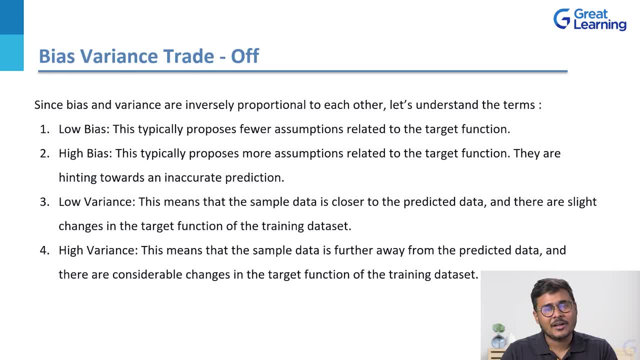 data and there are slight changes in your target function or the target data of your training data set, the training data set that you are using to teach your machine learning model. However, high variance means that the sample data is very far away from your predicted data. 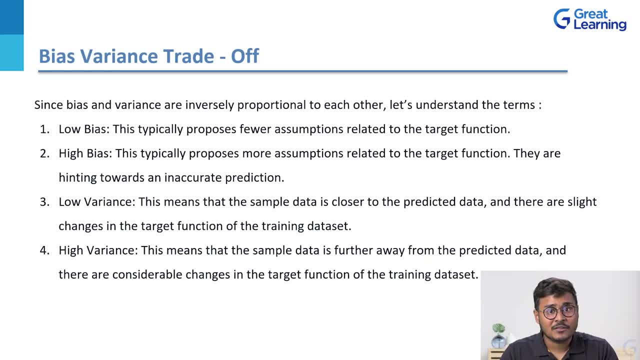 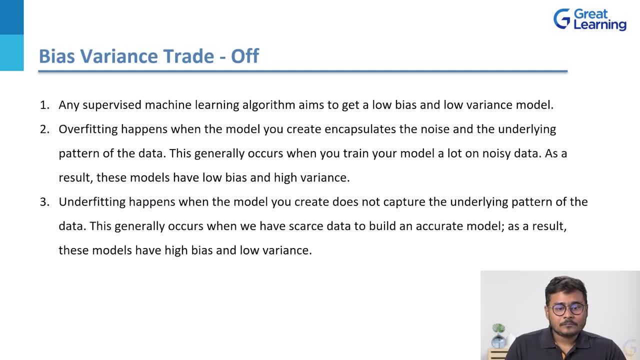 and you need to make a lot of considerable changes in your machine learning model of the or the target function of your training data set. Now let me move ahead and explain you about overfitting and underfitting, and then I'll also be drawing a graph so that you have a better 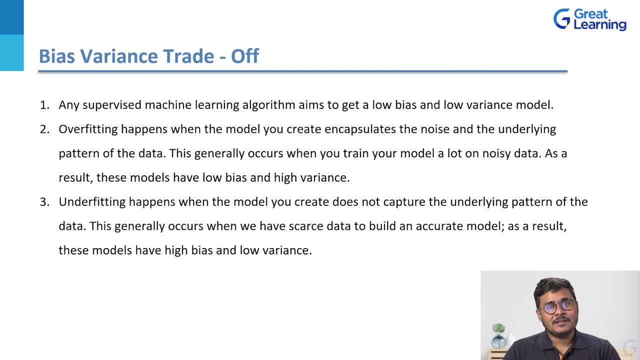 idea of both these terms. Any supervised machine learning algorithm aims to achieve high variance in your training model. So, for example, if you have a machine learning model, it always aims to get a low bias and a low variance model. However, in practicality, 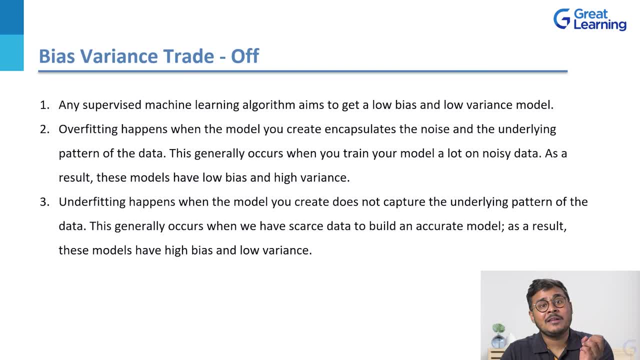 in real life you wouldn't find any ML model with an extremely low bias and low variance. That is practically not possible. Overfitting happens when the model you create encapsulates the noise. What do I mean by encapsulating Here? encapsulate means captures the noise and the 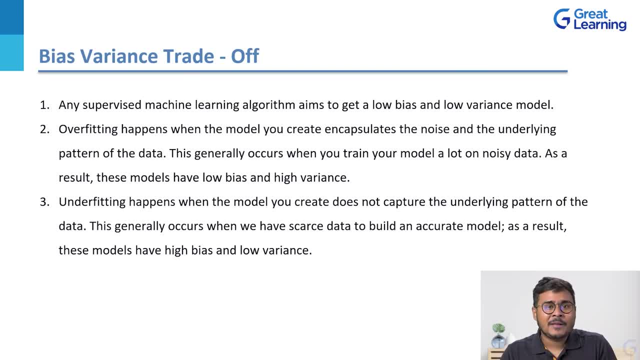 underlying pattern of the data. So this generally takes place when you try to train your machine learning model On a training data set which has a lot of noise. As a result, these models have low bias and high variance. However, underfitting happens when the model you create does not capture the underlying 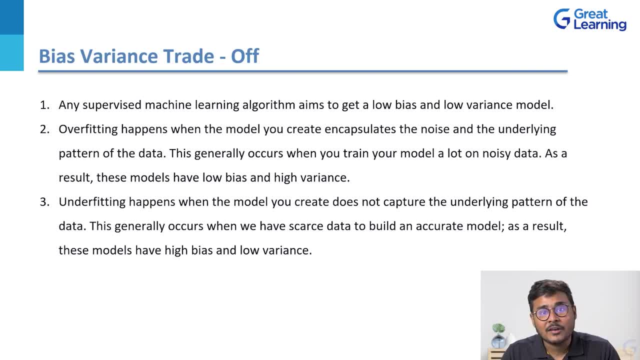 pattern of the data. So this generally happens when you're trying to train your machine learning model on a data set which has very small amount of data, or you can also say scarce data. As a result, these models have high biases and low variance. 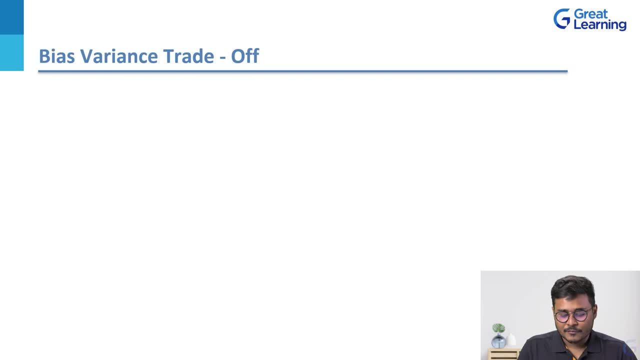 Now let me explain You overfitting and underfitting using a graph. So firstly, I'll start off by explaining you overfitting. So, as I told in the theory, we'll have a X and Y axis and we have the data which is spread across these axis, right? So let me just 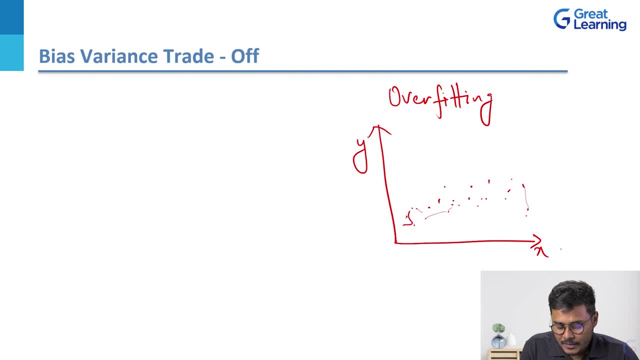 draw the points here. Here you will see that the lines are not eventually connected like. the data has a lot of noise, Also means that there is high variance and low bias, And as I've already explained you what overfitting means. So this is how an overfitting looks like on the graph. Now let me move forward and talk to you. 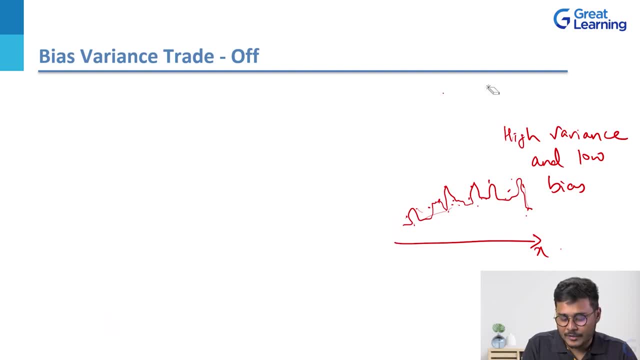 about or explain you or draw the graph of underfitting. In underfitting, we have the X axis and the Y axis, But here what we are having is, again, you have the data points, which is spread across both the per lower or lower axis, but we basically have a straight line which indicates towards having a high. 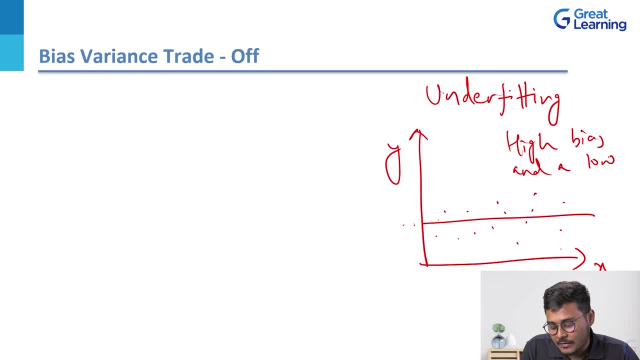 tutor, lessed by the target data type and a low variance. So, as I have explained you, what is overfitting for a data set is bla pok. but basically your sample data or your target function for your data fell lower and that is ever closer to your predicted data. So, in the example with you, when your data and your high phi. The value for these values is on to the X axis, But the number of times the data is overfitting, that means for the target function is close. So then your data, très large, is 0.025, then. 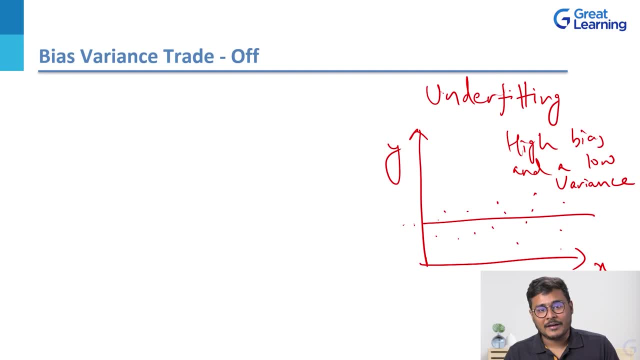 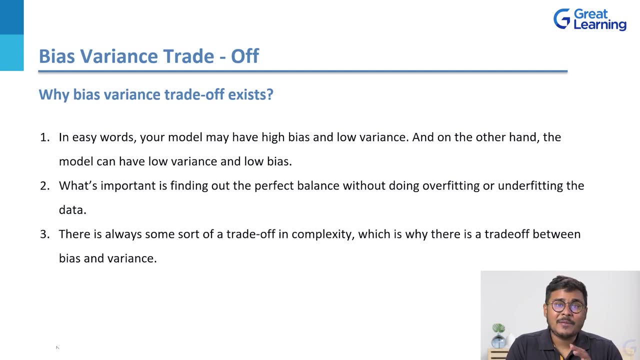 your data can only be push back when you have a path that is close to the target data type. As I have already, everything is high is when the underfitting generally takes place or happens. now let's move forward and understand the trade-off part right, so I'll be. 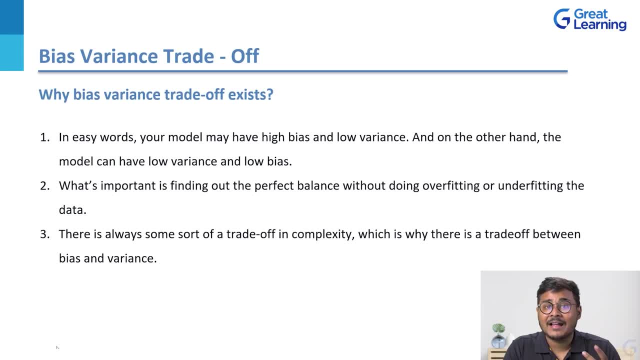 explaining this in two parts. firstly, I'll be explaining the why part of it, and then I'll be covering what is trade-off in bias and variance. so let me start off by explaining you the why part of it. in easy words, your model may always have high bias and low variance and on the other hand, your model can. 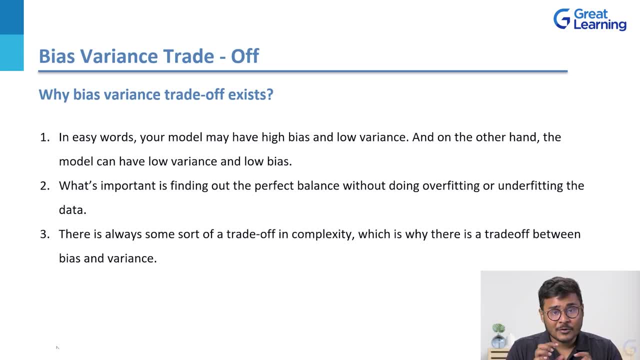 also have low bias and low variance. what's important to find out here is a perfect and optimum balance without doing overfitting and underfitting the data, and there that is a reason why there is always some sort of a trade-off- that exists in your complexity of algorithm- between the bias and the 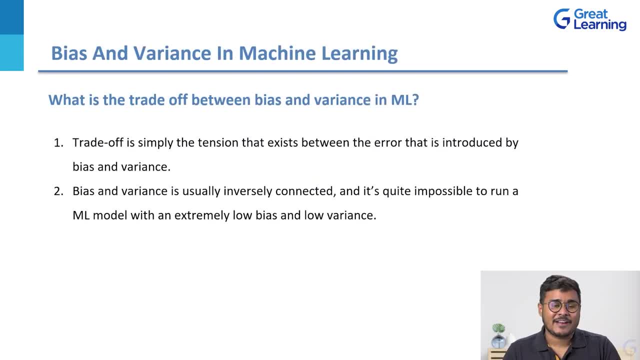 variance. now I'll be explaining about what is this trade-off? well, this trade-off is simply the tension that exists between the error- that is interesting- and the variance, and the variance, and the variance and the reduced by both bias and variance, since bias and variance are inversely. 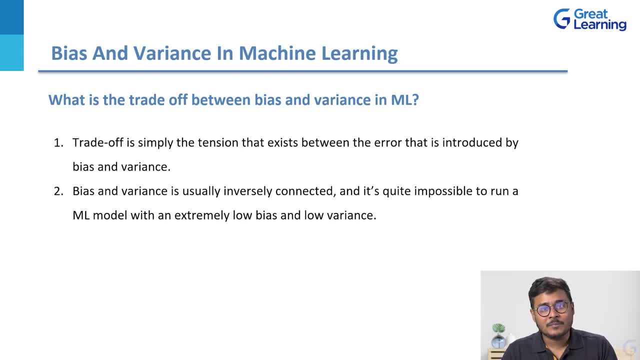 connected to each other. it's always quite impossible- and, as I had already talked about it, it's impossible to run an ML model with an extremely low bias and a low variance, so you might expect one of the other parameters to be high. what we try to do is minimize the error, and this is where the concept of total 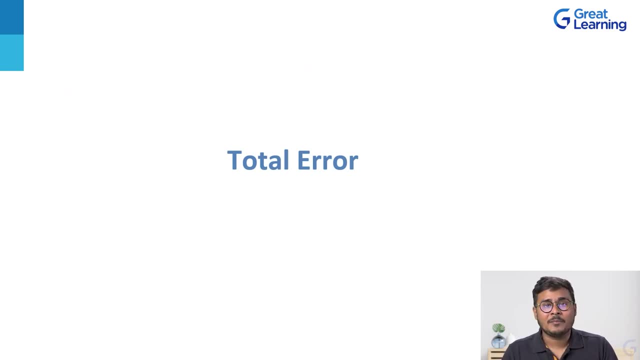 error comes into picture. in order to have a very optimum, perfectly balanced data, we need to minimize the total error between bias and variance. so what is this total error? well, this is all about finding the right balance between bias and variance, and we need to reduce or minimize this total error. and a right 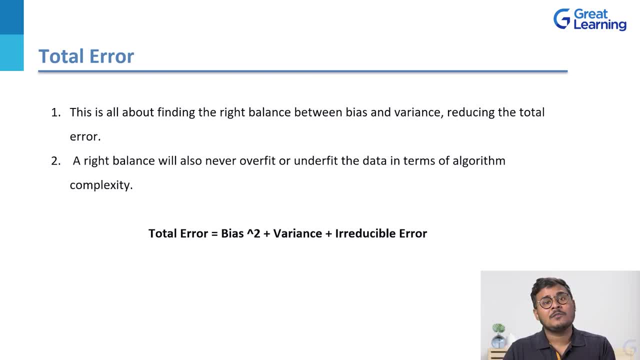 balance will never overfit and under fit the data in terms of its algorithmic complexity. so, as you guys can see, this is also the mathematical expression for total error here. so I've already explained what is the total error and what do I mean by irreducible error, when I started the presentation and about 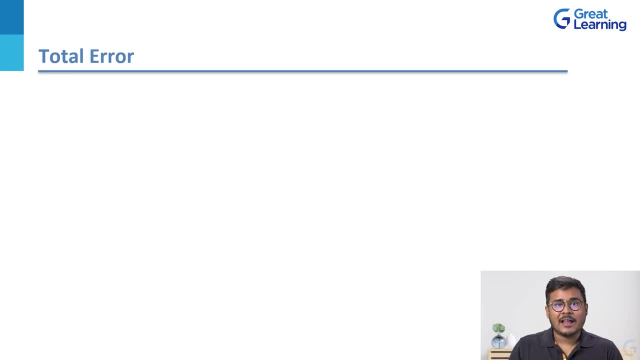 variance and bias. Now let's move ahead, where I'll be drawing the graph of total error, since it's always about finding the optimum balance right. So now I'll be drawing the graph, or the diagram, for total error. So on the x-axis, I'll have 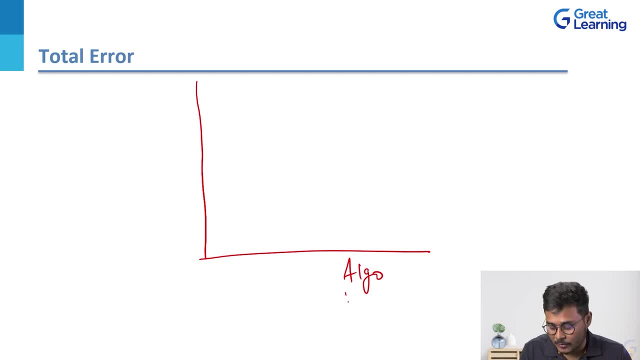 algo complexity, which also means algorithmic complexity, and on the y-axis I'll have error. So this is about. this is also called as optimum. I'm sorry, I think the spelling is wrong, So let me just erase it and write it again. So this is: 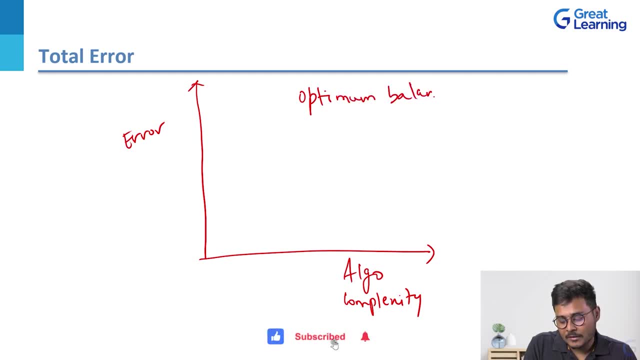 called as optimum balance. Now, how do I know that I have the optimum balance? How do I draw the variance and bias on the total error? so, if I have to show you in a very simple term, This is the intersection point where both bias and 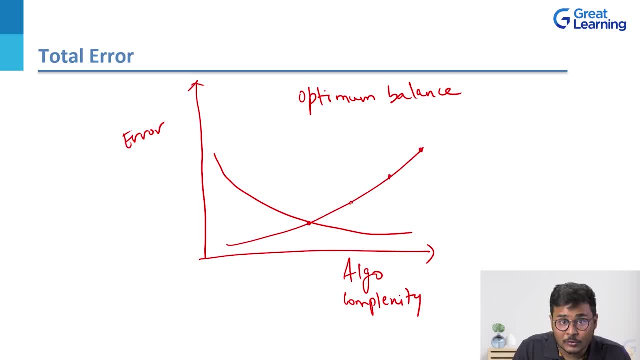 variance meet, and there are different data points here on both of these lines. right, so it starts from here, it goes here, also goes here, there, there and there. So this is your bias, cap 2, and this is your variance, and this is the part which is called as your total error, right? so since here we are trying to 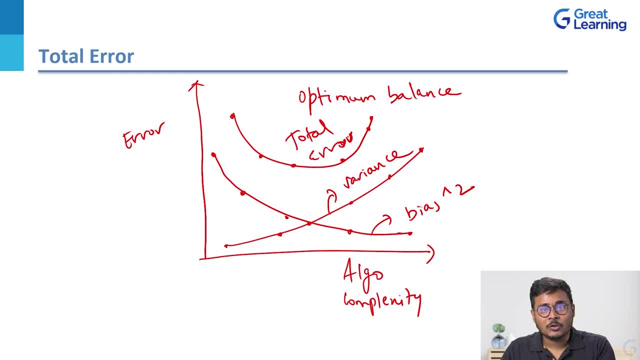 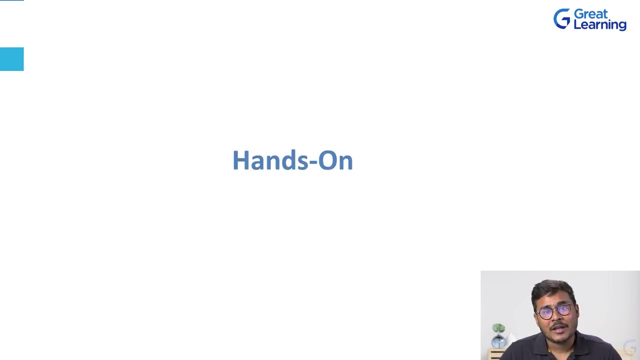 reduce or minimize the total error. so we are basically trying to achieve an optimum balance, and every time, whenever we want to make a good ml model, we always strive for minimizing the total error. so with this, let now let's move on to the hands-on part. here i have taken a diabetes data. 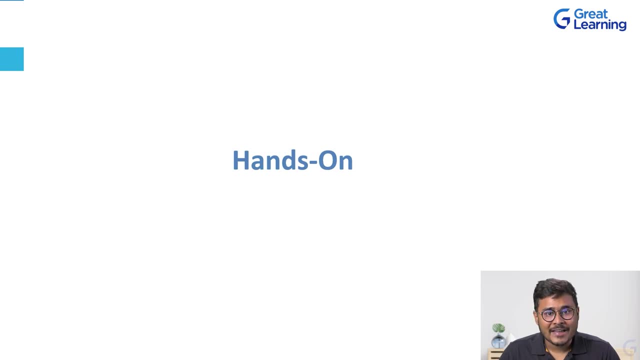 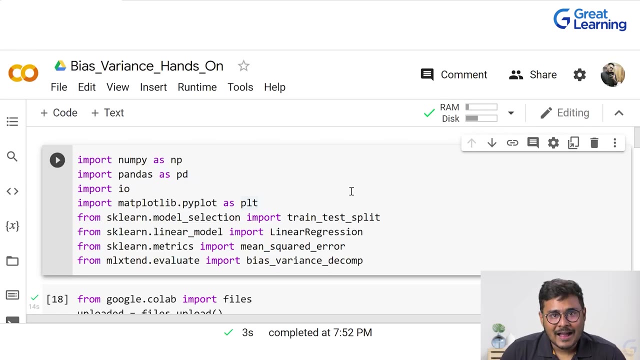 set, where i'll be showing you mean squared error, bias and variance error on that data set. so let's get started with the coding now. let me start off the hands-on, so here i'll be practically implementing the coding right. so what i have done is i have taken a data set which is already. 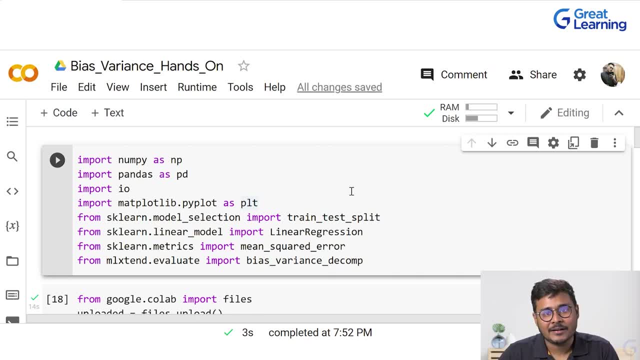 existing, and then i have tried to tinker with that data set a little and try to apply bias and variance. as you can see, the first two steps remain the same. i'm importing numpy as np and pandas as pd. i don't really need io here, so i don't think i'll be doing it. so i don't really. 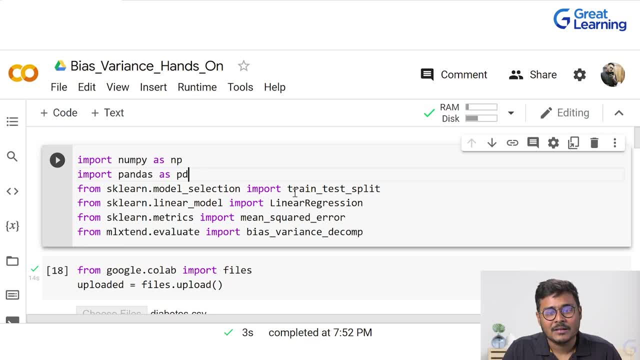 need matplotlib also. then i'm importing sklearn that is going to divide our data set into train and test split. then i also need to do linear regression here and i have to find mean squared error with bias variance decom. so what is this package, guys? do you see something different here? 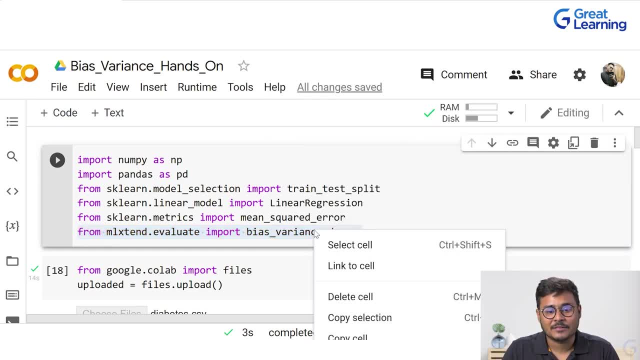 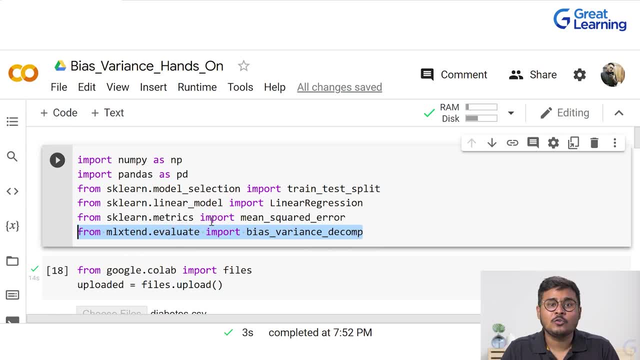 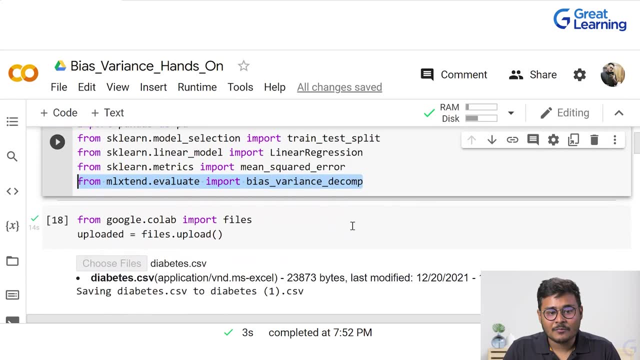 this is one of the packages offered by python to do machine learning activities or daily data science tasks, in a very easy way. as you can see this when i when i imported this part, this is going to make our coding life very, very easy, in spite of us writing a lot of routines and functions. 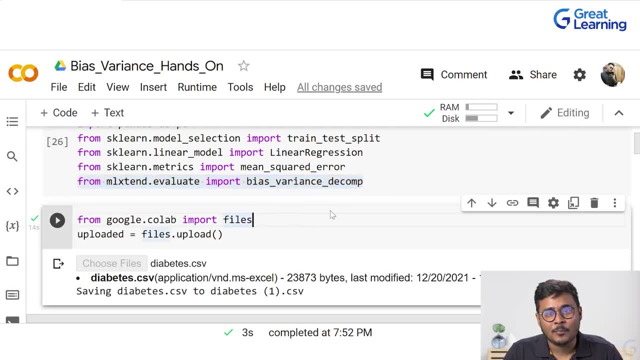 so as i move ahead, since i'm coding in google colab, i have to import the file. so these are the two lines of code that i have to import and i have to import the file. so i have to import the. i always have to write right, so let me just run this code quickly. 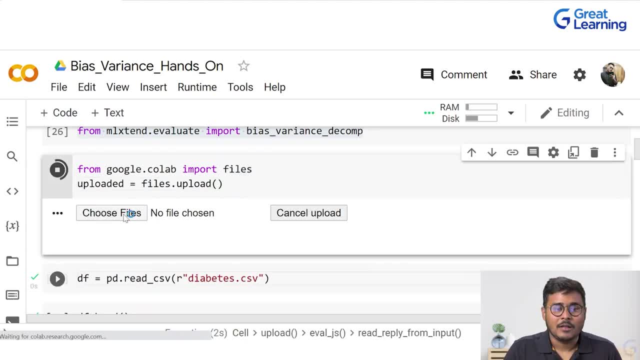 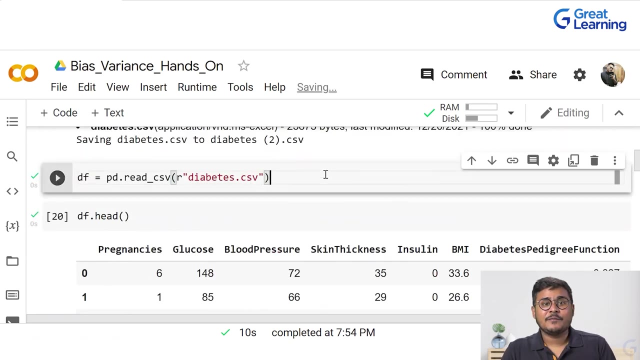 right now i'm going to choose my files. so i'm going to choose my file, which is the diabetes data set. i chose my file right and then i move forward. now i converted this diabetes data set into a csv file and i stored it into the df. so df is just the name or another variable name that i 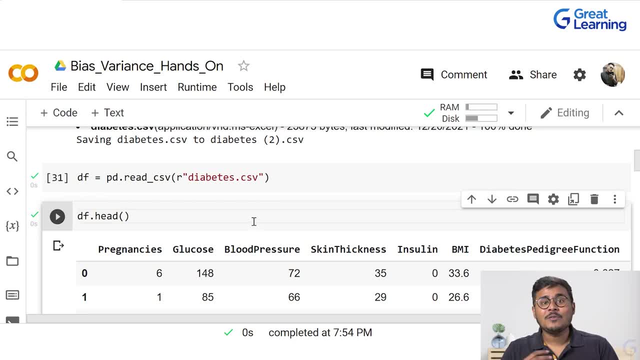 have given to store my csv files into. now i want to store my csv files into my df, so i'm going to. i want to understand what is the this data says. i want to see what this data set is about. for that i have written, in order to see the first few rows, you know i have written this function or this code. 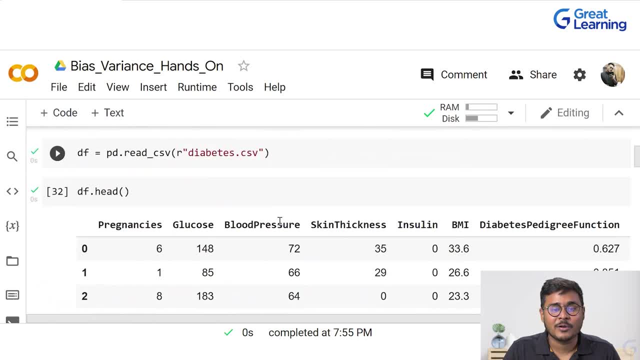 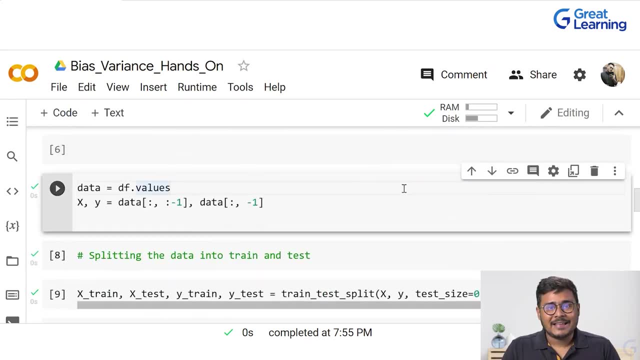 dfhead. so what is dfhead is going to fetch me? well, it is going to fetch me all the column names which are existing and the first five rows right now. we'll move forward and then assign this dfvalue. so i want to understand how the values look like, and then i have named two new variables here, which 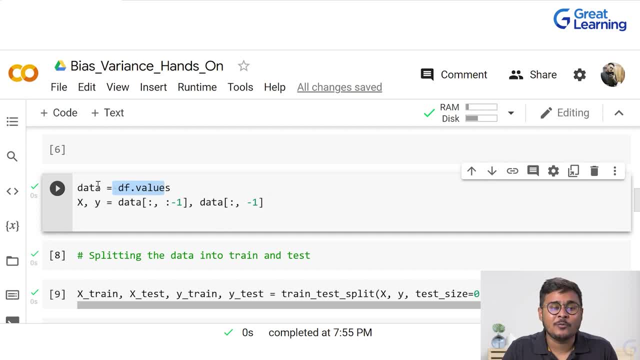 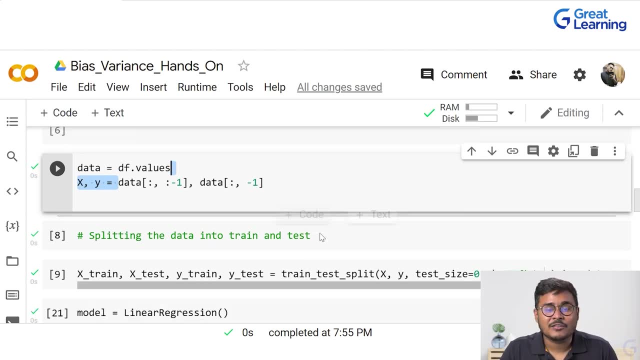 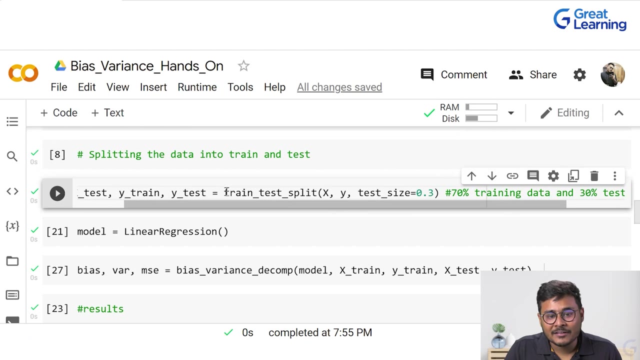 are x and y. so, firstly, i have assigned dfvalues into an entirely new variable, that is data, and then i'm slicing this data according to x and y, which also leads us to our next step, where we are splitting this data into train and test. so, as you can see the code for yourself when i'm writing, 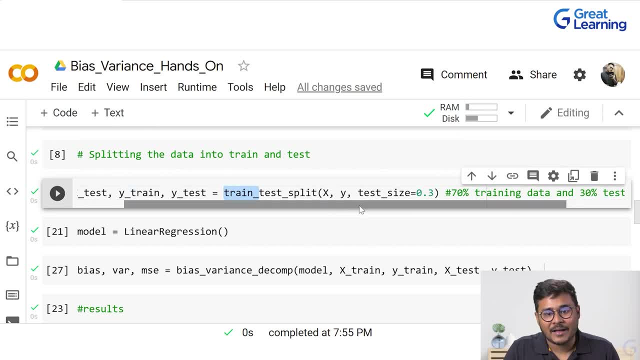 the code for train and test split. i have written this as x- y and the test size i have given as 0.3, which is the optimum way whenever you do write code for data science or machine learning, right? so you basically try to do it on 70% of the time, and then you have to do it on 70% of the time and 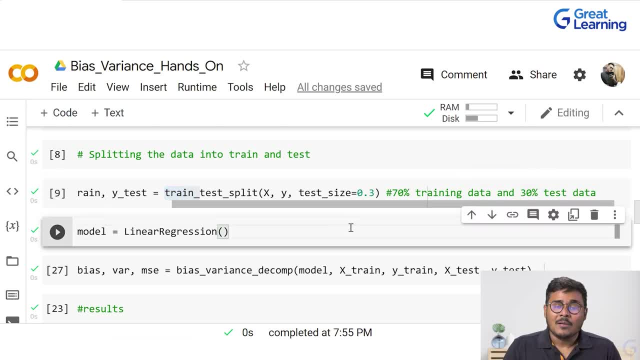 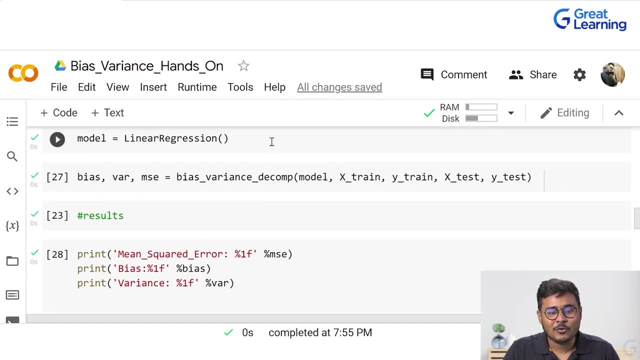 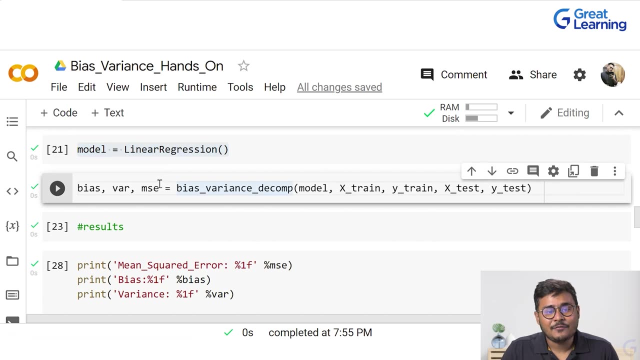 30% of the training data and 30% of the test data. moving forward, as i had imported the linear regression package already, i am basically creating a new variable where i'm calling the linear regression function right, so i'm invoking that function, which is an inbuilt part, and then finally, 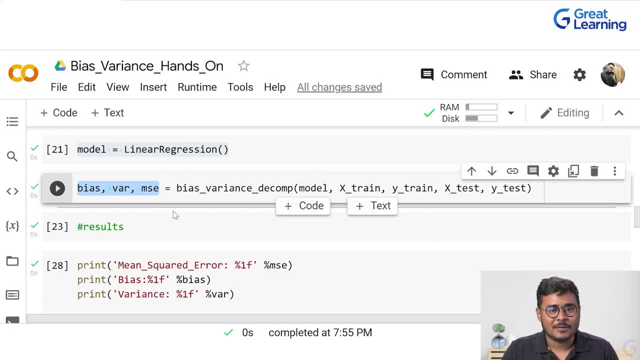 what i'm trying to do is i have named three new variables which are bias variance. the short form for variance is var, and then mean squared error, the short form is mse. and then, finally, what i'm going to do is i'm just writing the same code which is bias variance, decom. so do you see, guys? 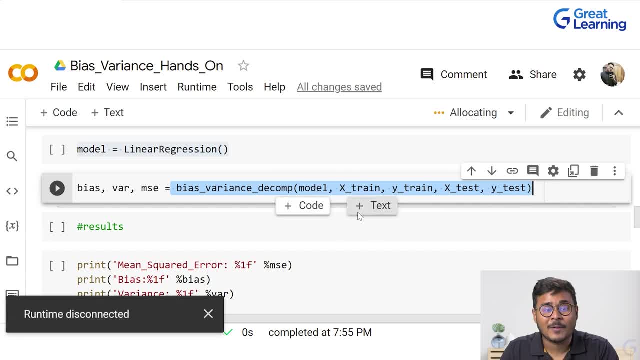 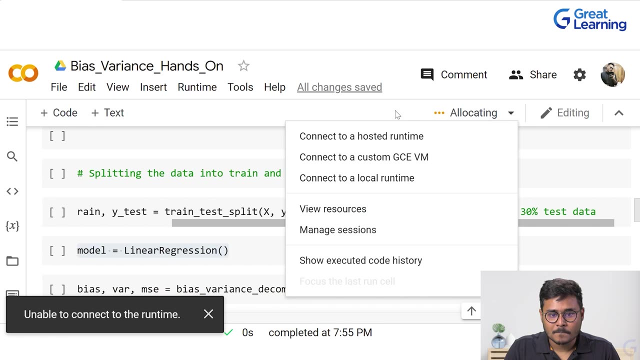 how your life has become so easy. now, it's just one line of code, in spite of you writing so many routines and functions prior to this, right. so you write this one line of code, you implement this in your model, right, and when you move forward- okay, i think it's reconnecting. yeah, okay, all right, so i 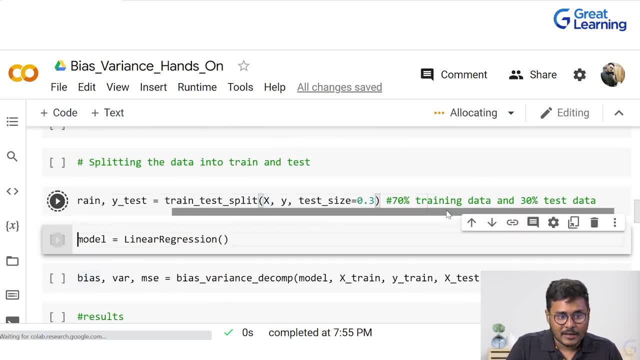 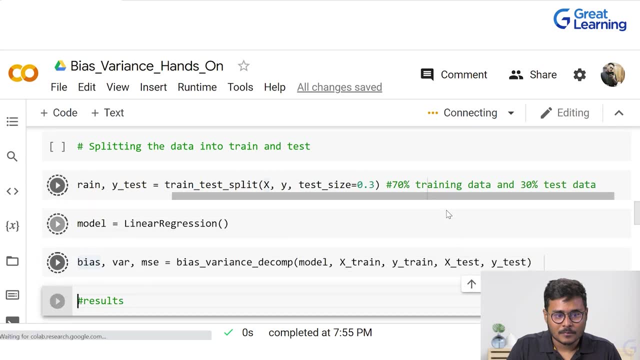 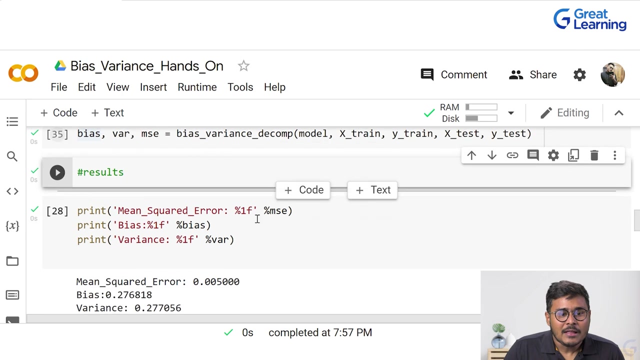 think i it's. it's sort of reconnecting here, but it's okay, i'll just run the code accordingly. it's it's connecting right now. okay, now it's connected. so this sometimes happens when you're using google collab guys, right? so once you're done with this part, we move forward, and now we want to see the results. 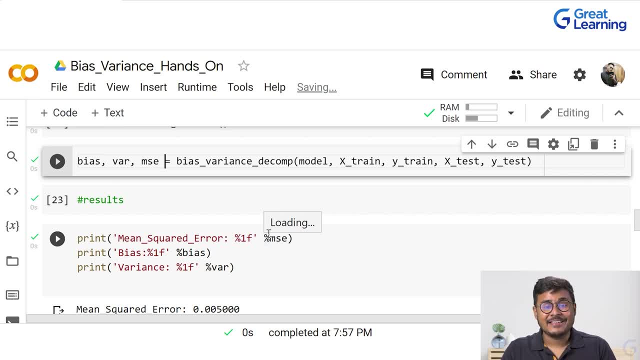 directly. now, guys, can you see how your life has become really, really easy? so you just wrote one line of code and you can actually apply and see what is the bias, what is the variance and what is the mean squared error of your data set right? so i just wrote this code. 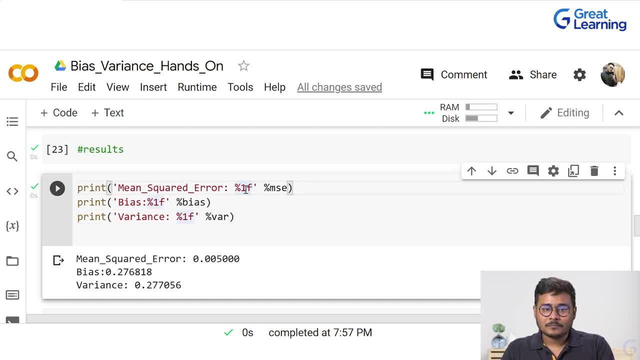 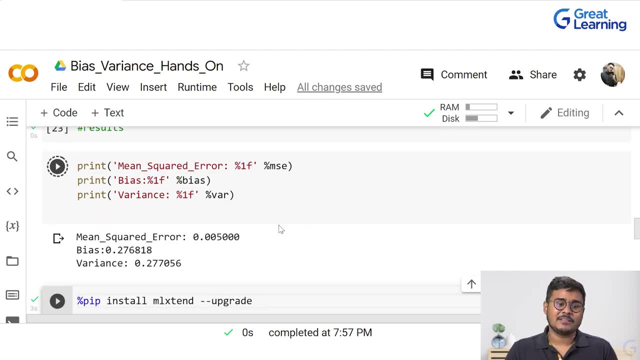 print your mean squared error with, you know, one decimal places to the right. you can use 2f or 3f also, just to keep tinkering with your code. and finally i received this result. so, as you can see for yourself, the bias is also low and the variance is low, but again, it is not extremely low. so this: 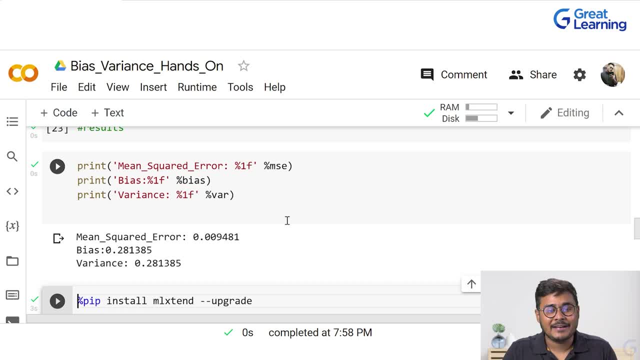 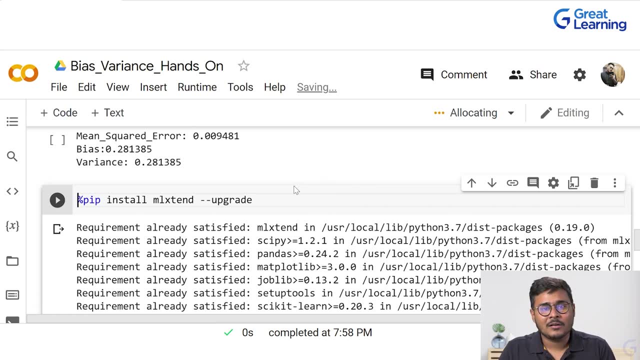 data is good to go. it is performing exceptionally well and you can see that the variance is also exceptionally well on our training data set also, guys, i want to end this coding tutorial, or this hands-on part, on one note: whenever you're trying to import this particular library, which is from 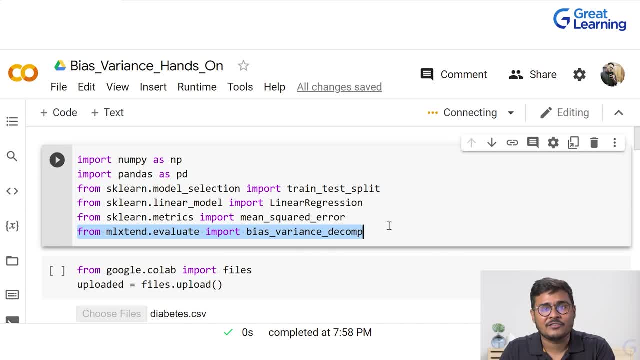 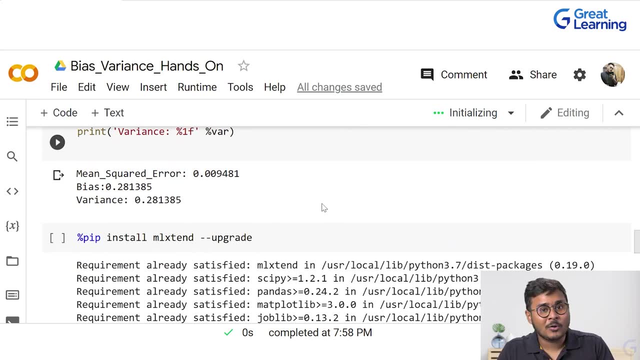 machine learning extension. it's called as a machine learning extension library or package. you need to install it first, and this goes for both of the people, so people who use google collab or people who use anaconda or jupyter, right? so you need to write pip, install mlx. 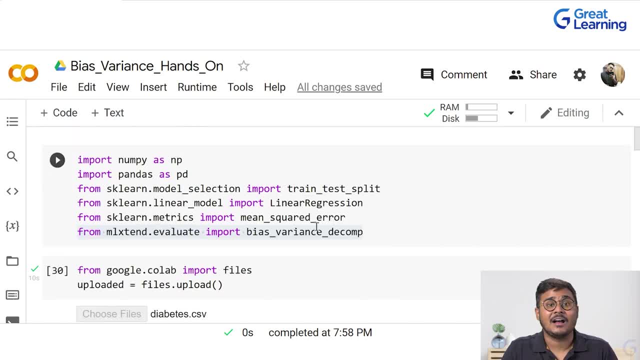 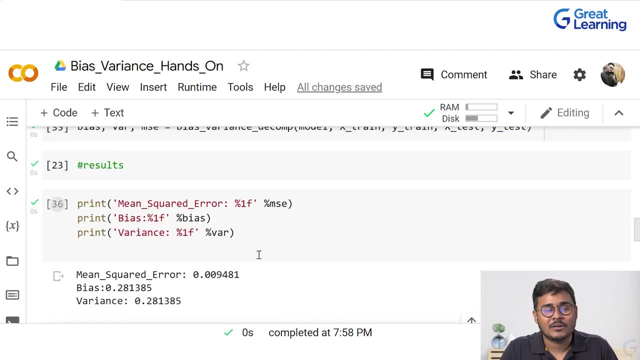 tnd upgrade and then you can use this package directly. otherwise it is going to throw you an error, since for me, even if i delete it right now, it is not going to throw an error because the requirement is already satisfied. so with this, guys, we come to an end of the coding session, or i can. 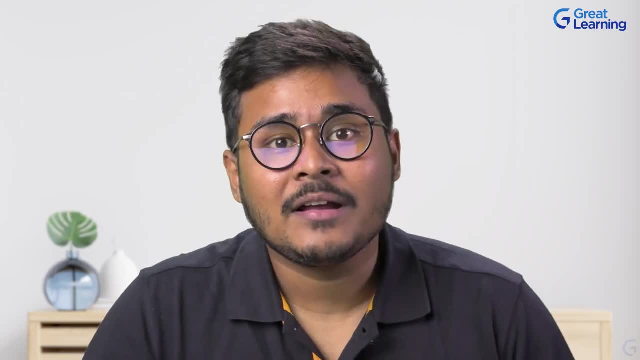 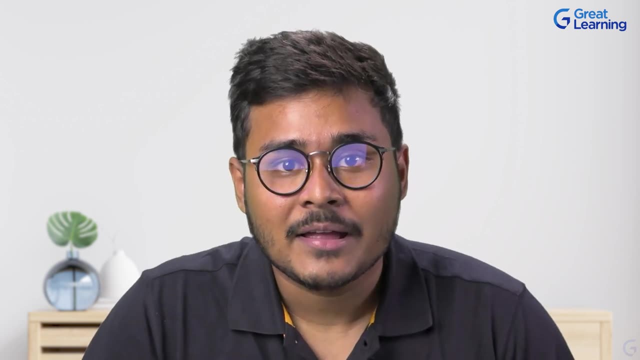 say the hands-on part. i just showed you the hands-on using a data set. now, with this, we come to an end of the presentation, so let me quickly summarize all the points that i covered in the entire presentation. so i started with the first part and then i started with the second part, and 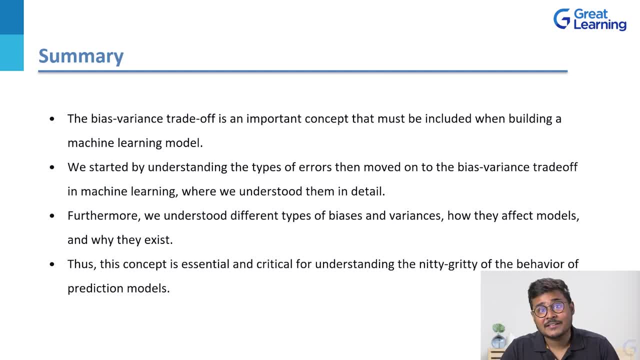 i started off by explaining you what is bias variance trade-off and why is it such an important concept that you know must be included when you are trying to build a machine learning model. then we understood the types of errors and moved on to the bias variance trade-off. so there were 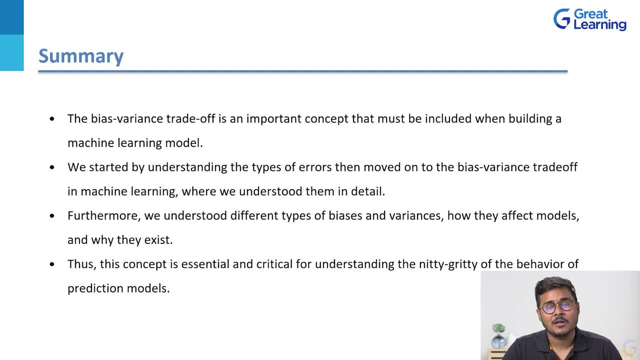 two types of error. one was irreducible error and the other one was reducible error. and when, then, we understood about the bias variance trade-off in machine learning in detail? furthermore, we also understood about different types of biases and variances, where i made you understand about two.